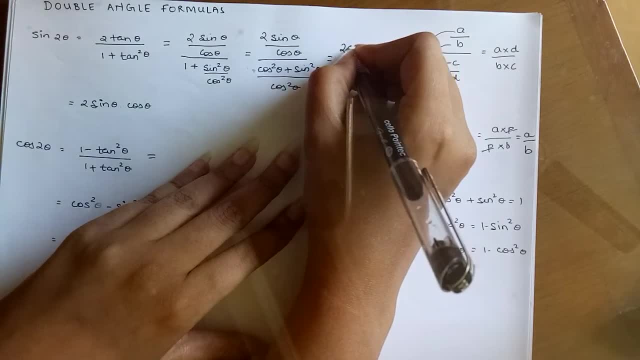 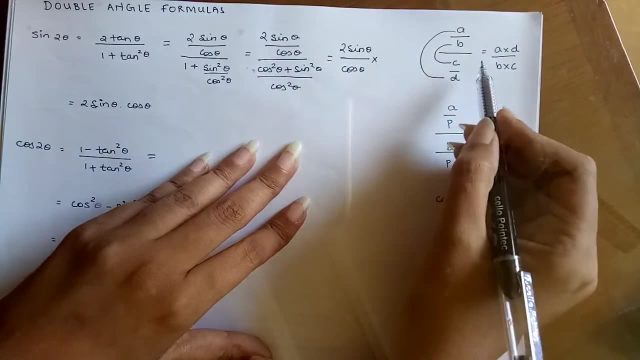 will be nothing but 1.. Okay, so I get tan square theta plus sine square theta will be nothing but 1.. So I get something like this: 2 sine theta upon cos theta. Now, according to this logic, my sine theta will get multiplied by cos square theta. 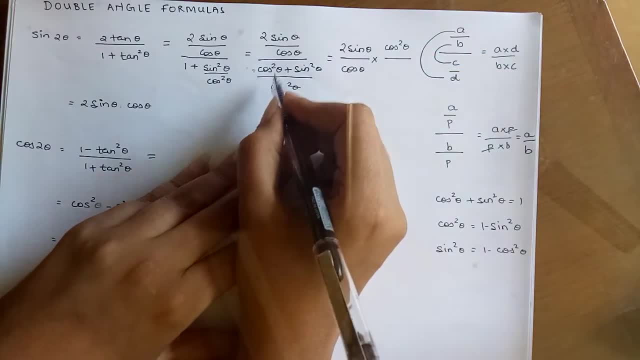 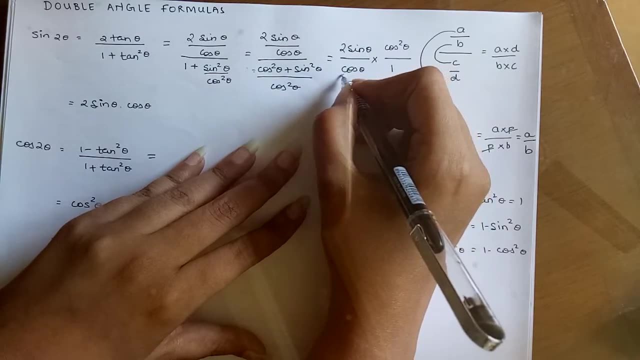 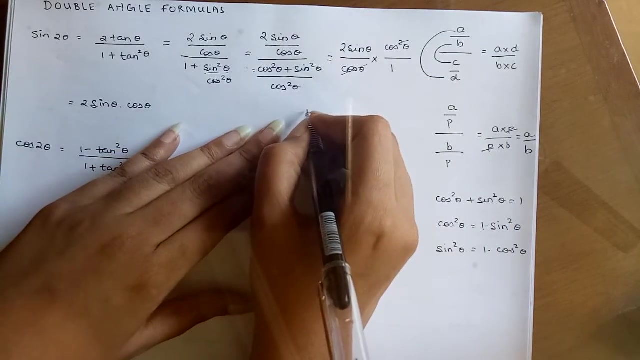 and cos theta will get multiplied by cos square theta plus sine square theta, that is nothing but 1.. So now my cos theta can get cancelled by the cos square theta in the numerator. So I get something like this: 2 sine theta into cos theta. 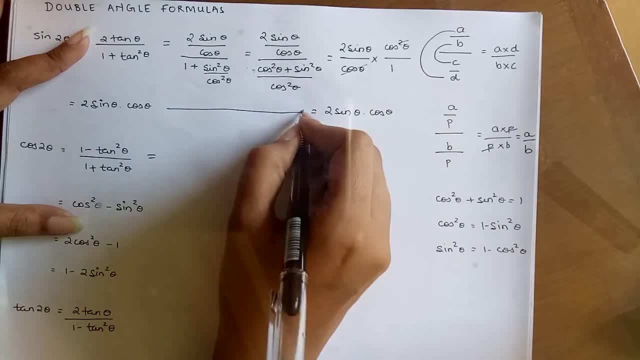 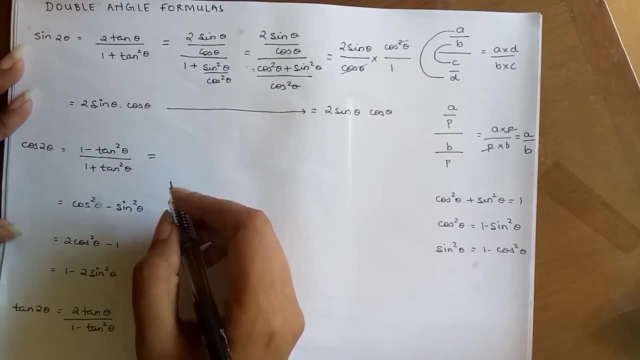 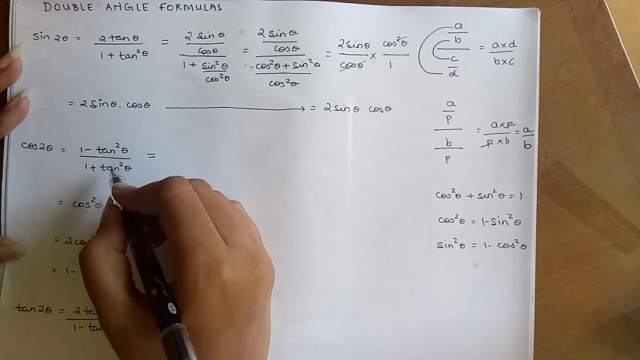 So in this way I have got my second formula for sine 2 theta. Now let's come to my next formula, which is nothing but cos 2 theta is written as 1 minus tan square theta upon 1 plus tan square theta. I'm just going to use the same logic where tan square theta can be written as sine square. 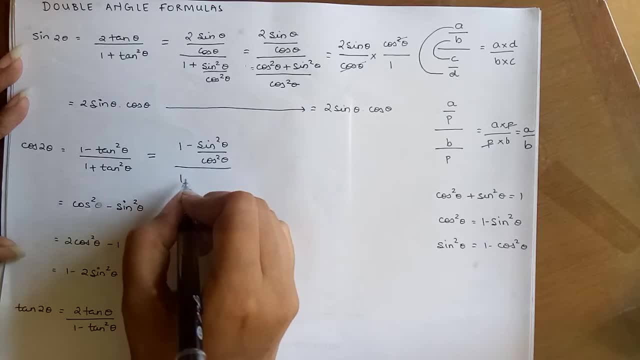 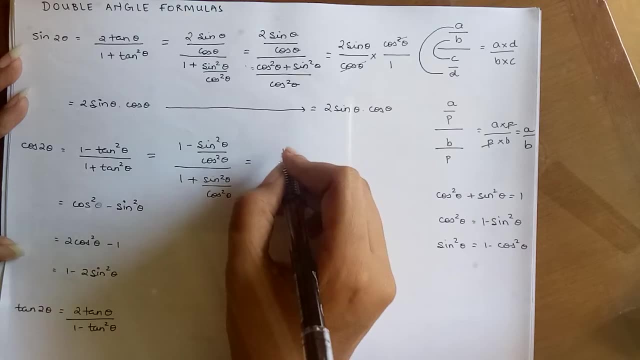 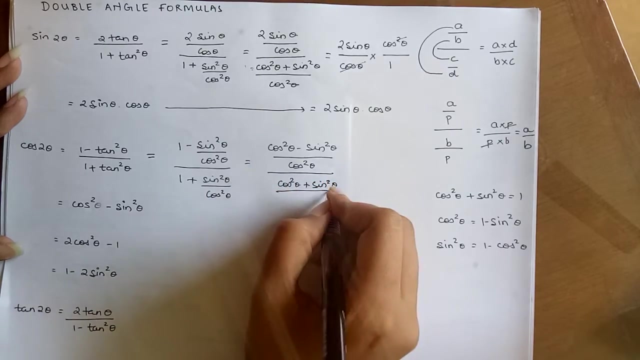 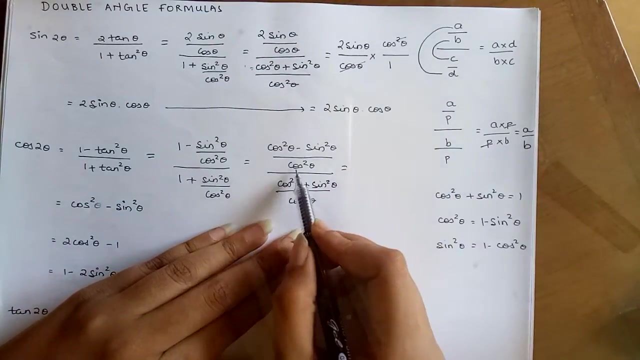 theta upon cos square theta. Now for my next step. I will just take LCM in my numerator and denominator, So I get cos square theta plus sine square theta upon cos square theta. Okay now, according to this logic, whenever I have the sine square theta, I will just take: 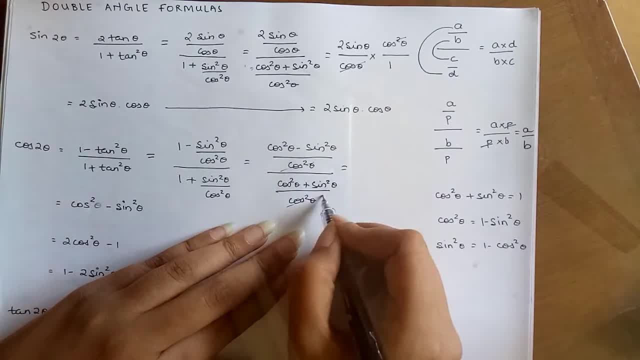 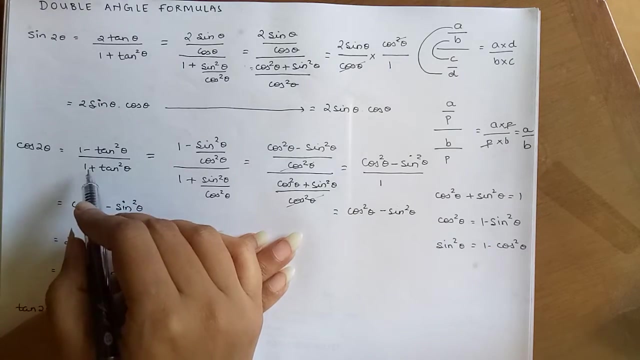 the same denominators, I can directly cancel them. So I will get cos square theta minus sine square theta upon cos square theta plus sine square theta, which is nothing but 1.. So I can say that my formula 1 minus tan square theta upon 1 plus tan square theta can also: 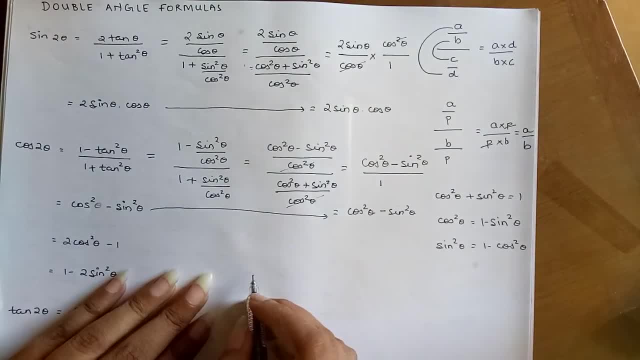 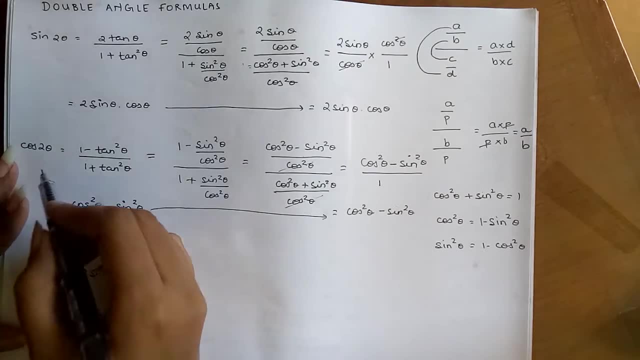 get me the next formula, which is nothing but 1.. So I can say that my formula 1 minus tan square theta upon cos square theta minus sine square theta. Okay now, as you can see that there are two other formulas for cos 2 theta. 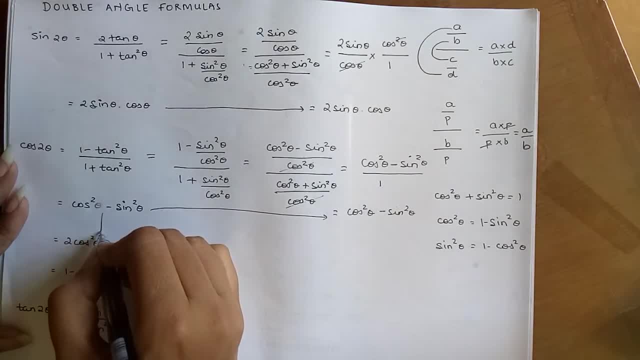 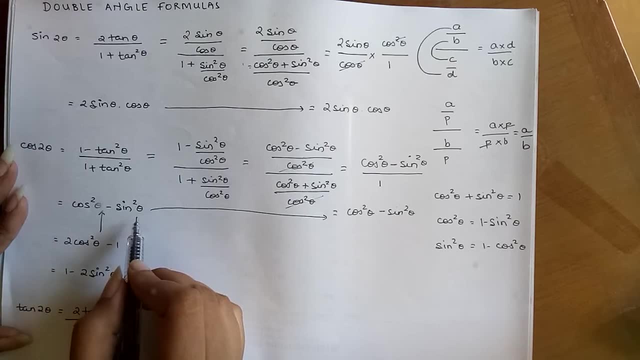 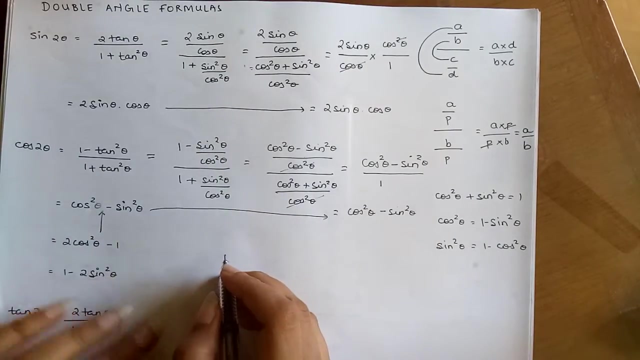 To derive these two formulas, I'm going to use this main formula. Okay, so now, if I want to represent this entire formula in terms of cos square, So I can write this sine square term as nothing but 1 minus cos square theta. So let me just write this down separately. 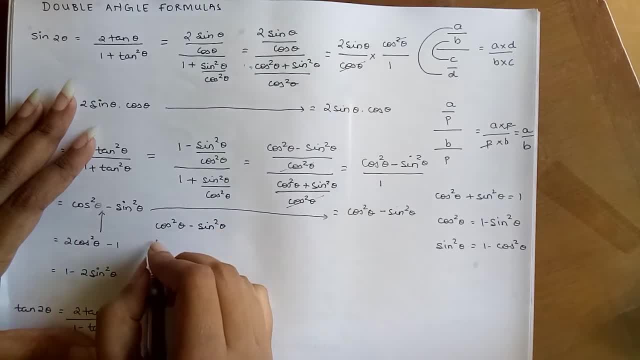 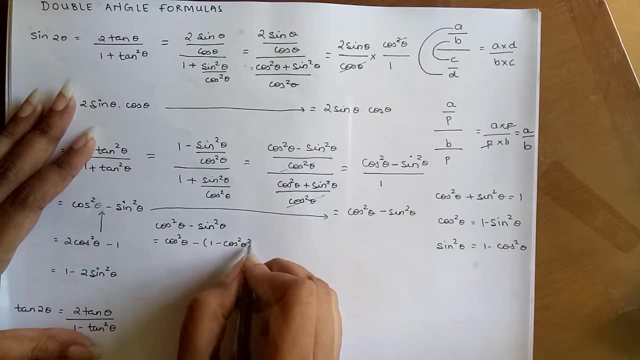 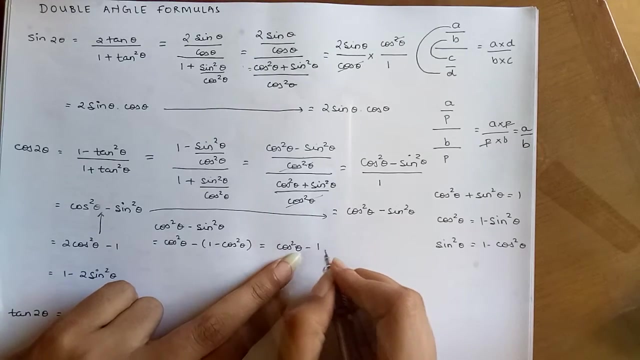 For you can be written as cos square theta minus 1 minus cos square theta, Okay, and when I open my bracket I get cos square theta minus 1 plus cos square theta, which is nothing but 2 cos square theta minus 1.. So in this way I can derive: 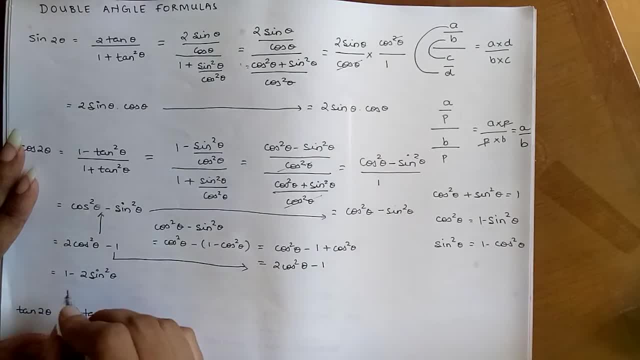 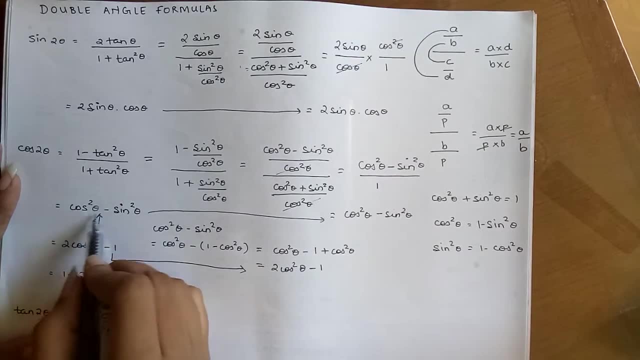 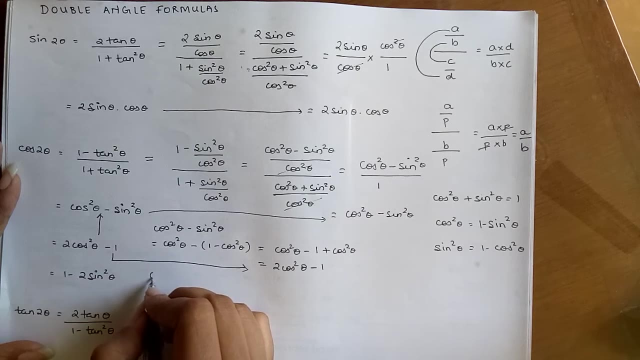 My third formula, Similarly, to express everything in terms of sine, I'm again going to use this formula, But instead of using cos square, I'm going to represent cos square theta as nothing but 1 minus sine square theta. So let's just write this formula again. 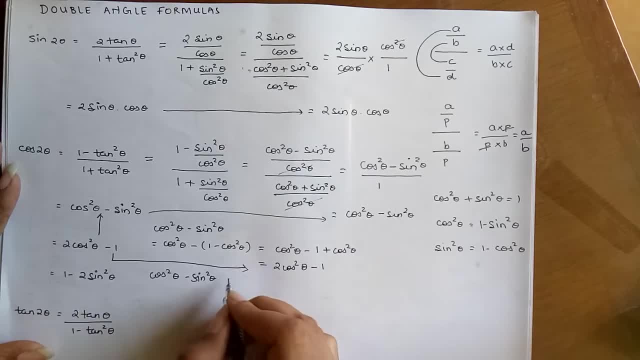 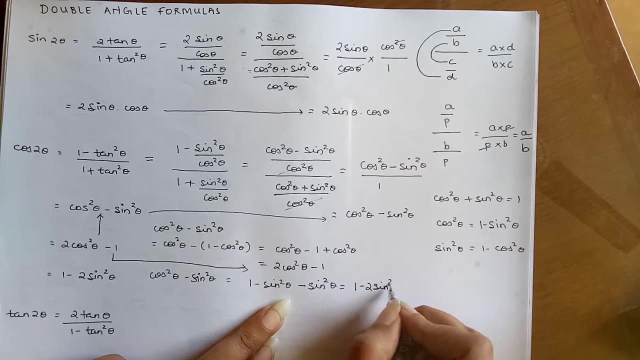 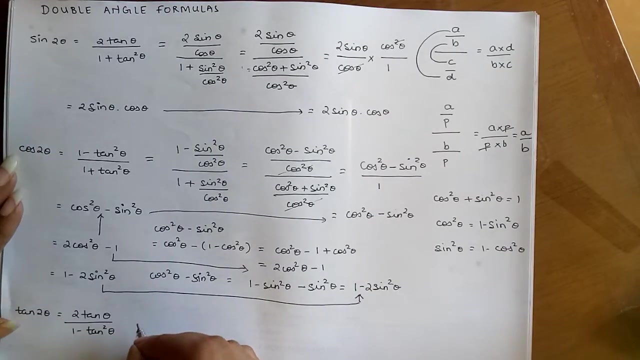 Cos square theta minus sine square theta, Where cos square theta is nothing but 1 minus sine square theta And the left over sine square theta. So this gives us something like this: 1 minus 2 sine square theta. So in this format I have derived my last formula for cos 2 theta. 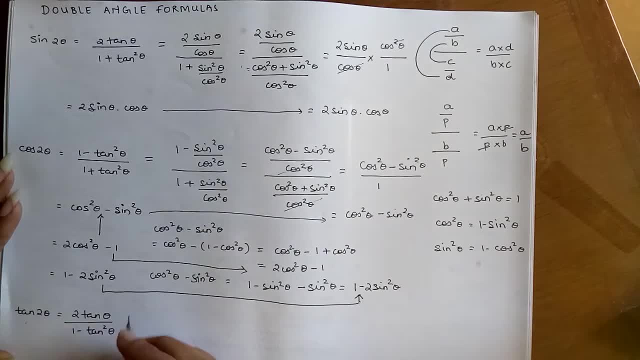 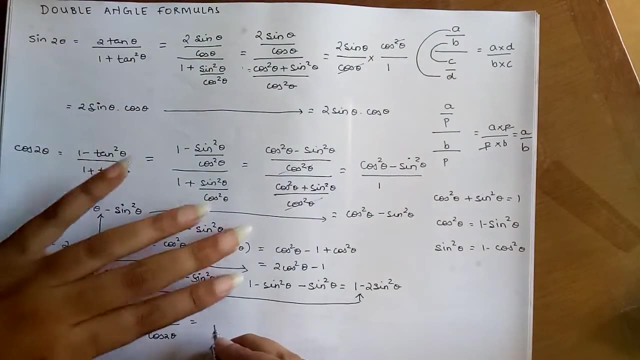 Now the last formula, which is nothing but tan 2 theta. As we all know, tan 2 theta can be written as sine 2 theta upon cos 2 theta, And And sin 2 theta is represented as 2 tan theta upon 1 plus tan square theta. So just let's write that. 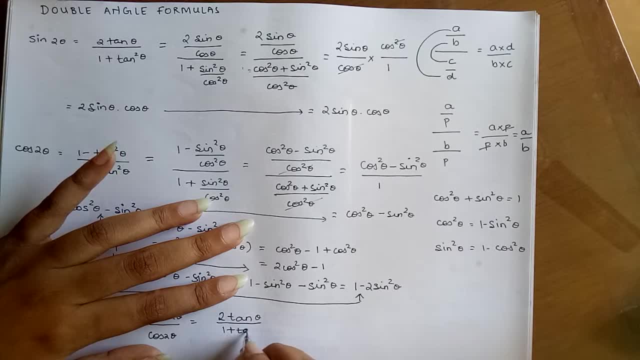 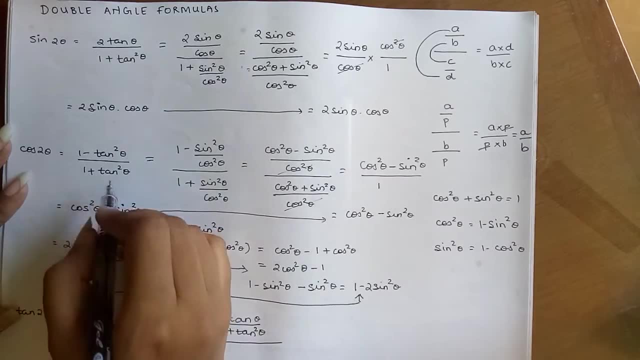 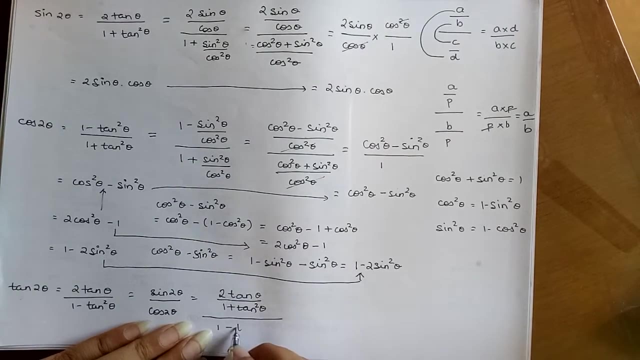 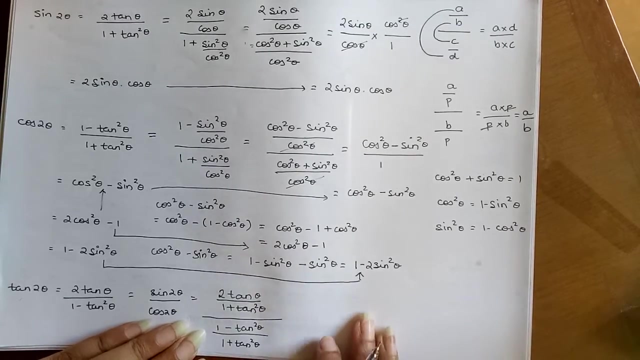 down this formula, which we have already remembered. Similarly, cos 2 theta can be represented as 1 minus tan square theta upon 1 plus tan square theta. Okay, as you can see, the denominators are same. So whenever we have a fraction over a fraction,